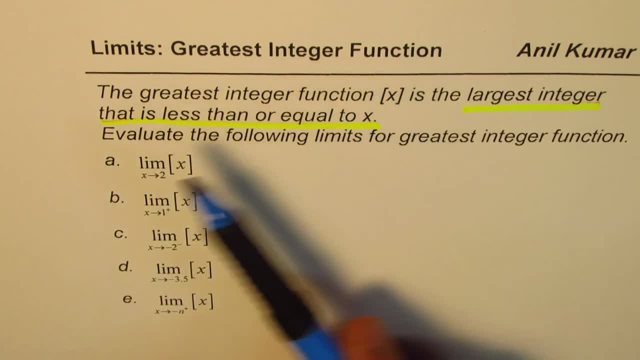 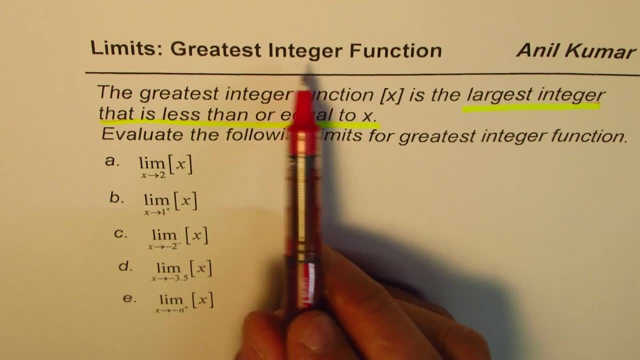 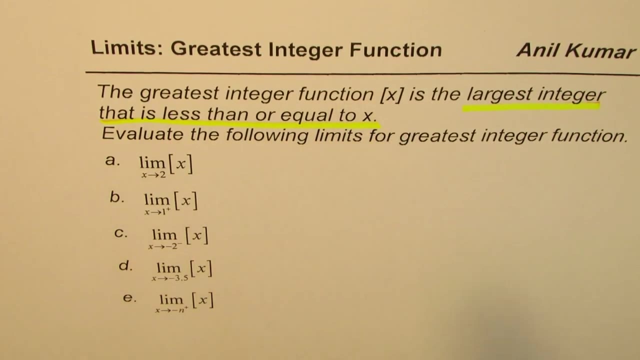 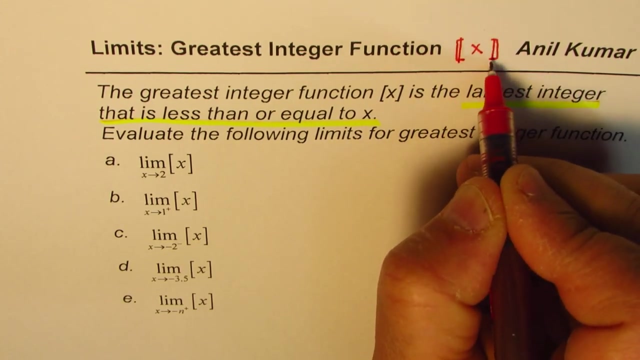 of what greatest integer function is, and then we'll solve a question based on limits. The question here is about greatest integer functions, which are defined as follows: The greatest integer function, and written as this. sometimes we also write them as these brackets, kind of double line on this side, So sometimes like this Now. so these square brackets, So the. 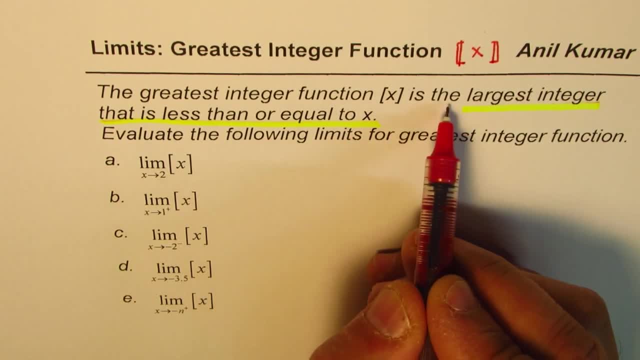 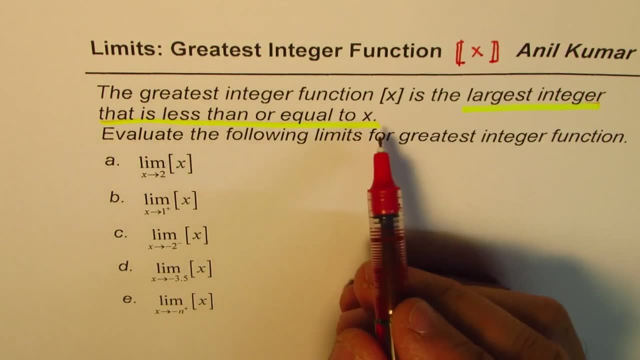 greatest integer function, which is written in square brackets, is the largest integer that is less than or equal to the greatest integer function. So the greatest integer function is less than or equal to x. That is how you define it, And what we need to do is to find the limit for. 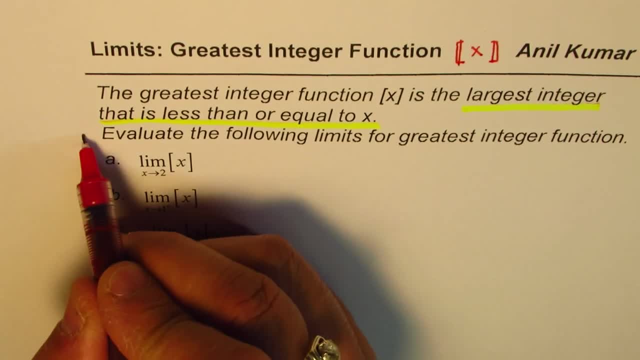 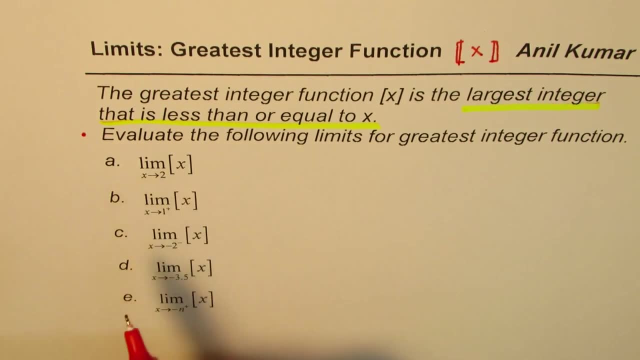 this function at different points. So the question here is: evaluate the following limits for greatest integer function Limit: when x approaches 2, when x approaches 1 from the right side, When x approaches minus 2 from the left side, When x approaches minus 3.5 and in general when x approaches. 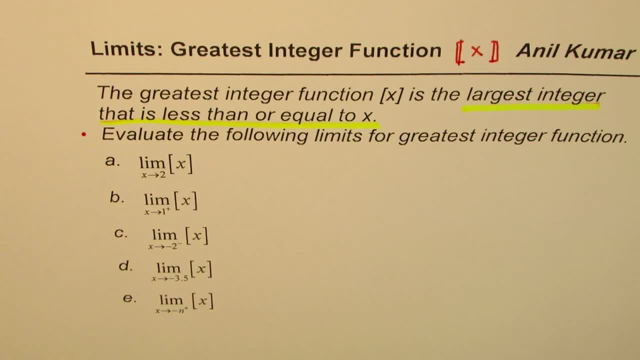 x approaches minus n from right side. So these are different limits which you need to figure out. Some of you can always pause the video, answer the question and look into my suggestions. Visualizing these values is kind of difficult, So what I will do here is sketch a graph to. 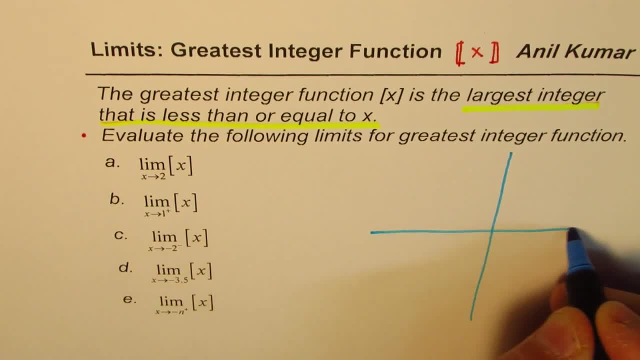 represent the greatest integer function, Right? And then we'll read the values from the graph. That's the whole idea. Okay, So to sketch the graph, let me pull mix. Okay, That's okay. So I'll make a rough sketch here. 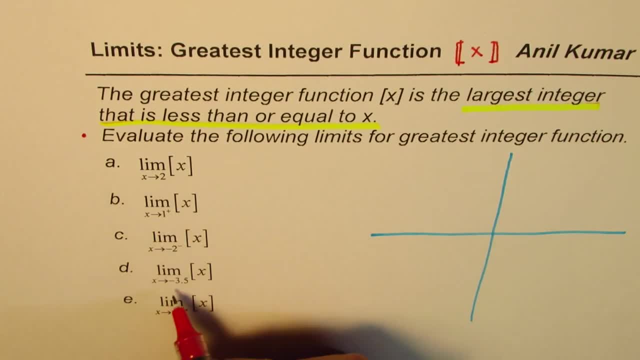 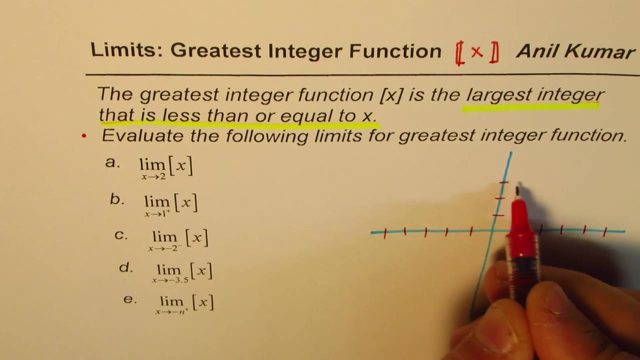 So we are interested in values from 1 to 4, basically Okay. So let me write down this is 1, 2, 3, 4, 5.. Minus 1, minus 2, minus 3, minus 4, minus 5.. Similarly, we'll do here 1, 2, 3, 4, and so on: Minus 1, minus 2, minus 3,. 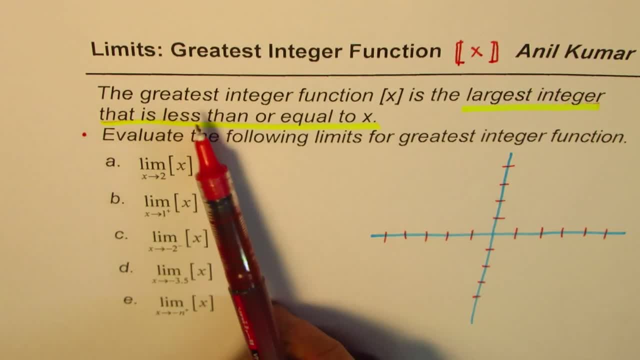 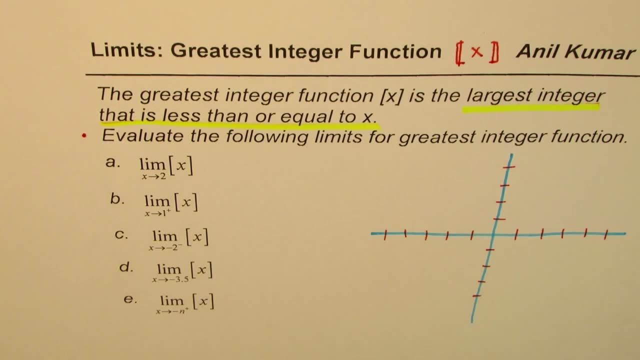 minus 4.. So, as you see, the definition is that the greatest integer function is the largest integer that is less than or equal to. So, basically, if the value is greater than 0 slightly, integer is 0. Right And up to, let's say, 1.999, it is 0. When it becomes 1, it jumps to value 1.. So it becomes 1.. 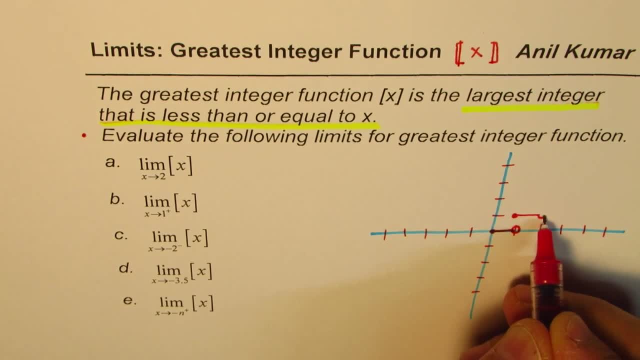 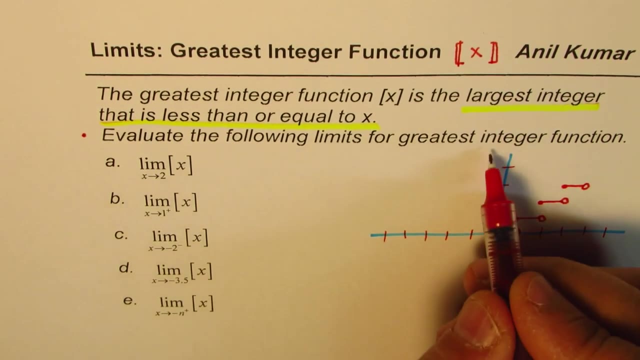 Integer 1.. And then when you increase up to 2.. So at 2 it jumps And then the same thing repeats. Do you see that? So that is how you could actually graph your greatest integer function, Right? So this is what we are doing. We are doing graph of greatest integer function Books normally use. 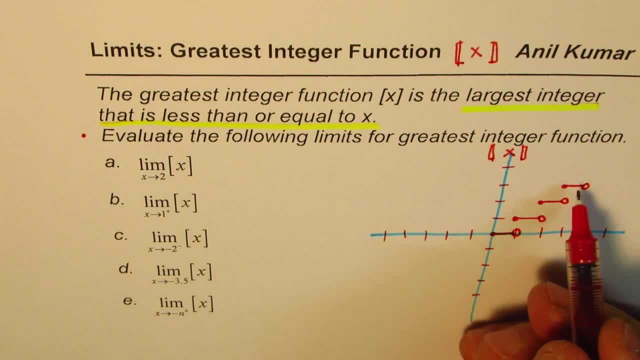 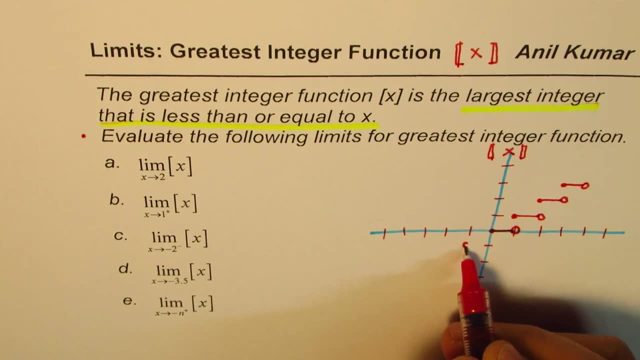 this sign. So I'm using the same. Follow this pattern. It's kind of difficult to understand for negative values. Just follow this pattern. I'm sorry to say that, But that's what I feel, You know, looking into response of students So, and then we'll try to understand why it is so. So we are just following. 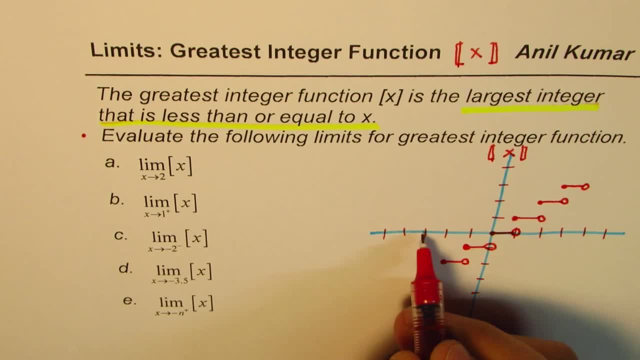 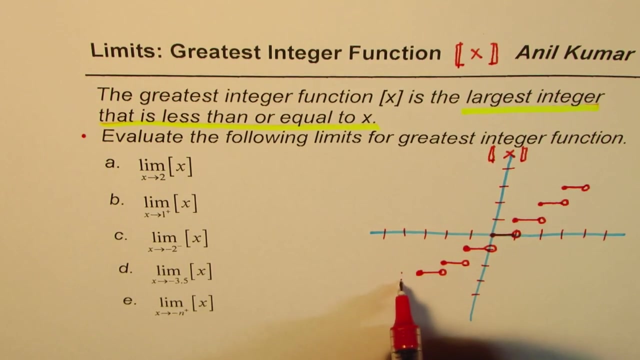 the pattern for the time being. So just be with me, And then we just kind of: do you see what I'm doing? So this filled in hole, or the circle is to the left side, And we are saying that left side or the number line is always lower Right. So less than Does it make sense to you? now I think it does Right So. So that is how it is. So it is kind of like this, OK, 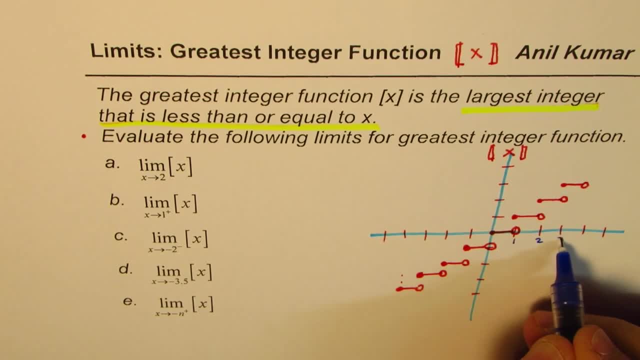 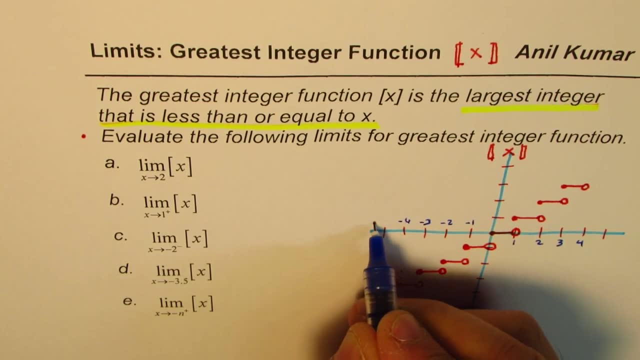 So we have some values here: 1, 2, 3, 4.. And this is negative 1. Let me write like this: Negative: 1 negative, 2 negative, 3 negative, 4.. We always break rules just for convenience, Right? 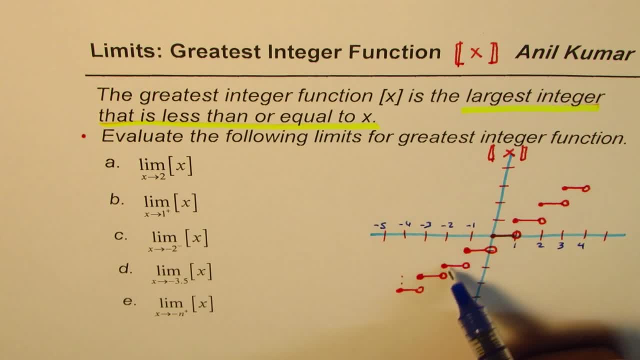 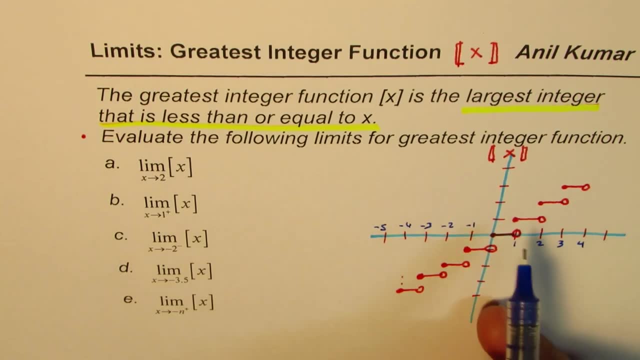 We always break rules just for convenience, Right. So for that I think sometimes it makes sense, because I don't want to mess with this side where we have the meat Right. OK, So now let's answer the question First one here is: what is the limit of the greatest integer? 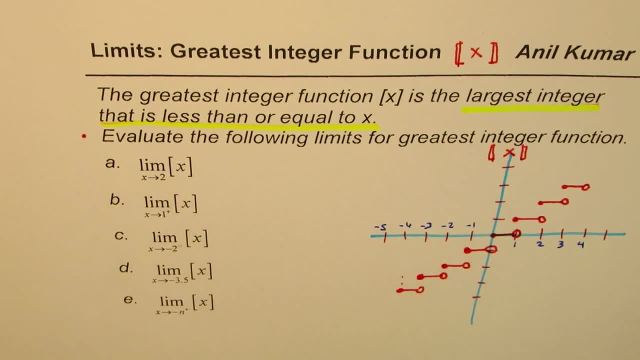 function when x approaches 2.. So when you are approaching 2, you could approach. You have to approach from both the sides, left and right, And you see, from left side it is approaching the value 1.. Right and from the right side you approach the value 2 and therefore this is: this is a 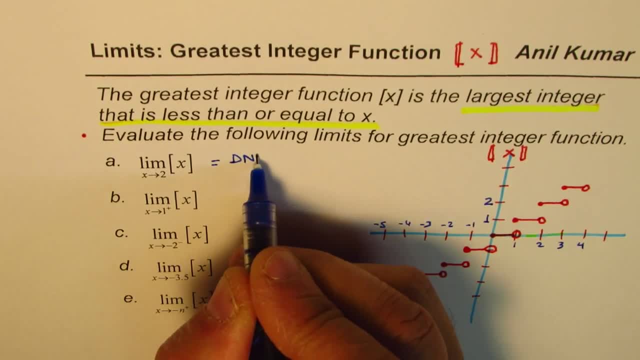 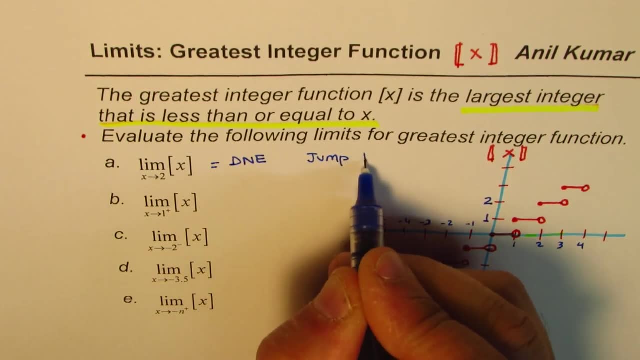 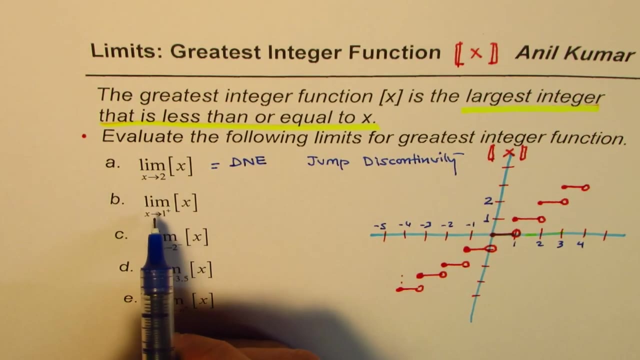 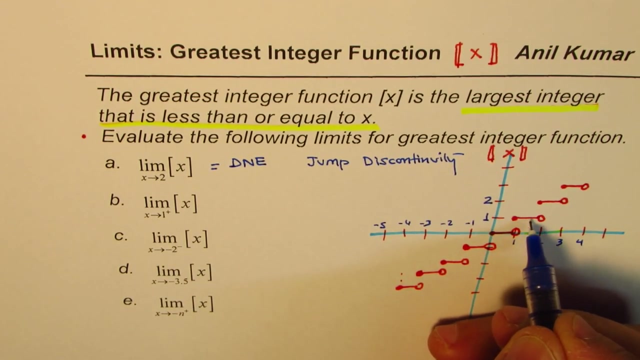 step function. there is a discontinuity. it does not exist, all right, so we have a jump discontinuity at this point. is that clear? okay, let's move forward now. we are saying limit of X when X approaches one from the right side. so we are approaching one from the right side. so you are on this part of the step and 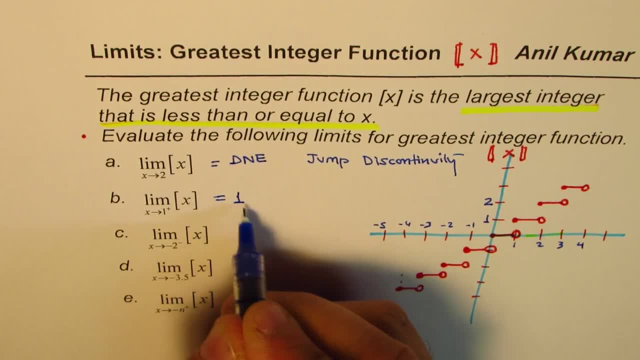 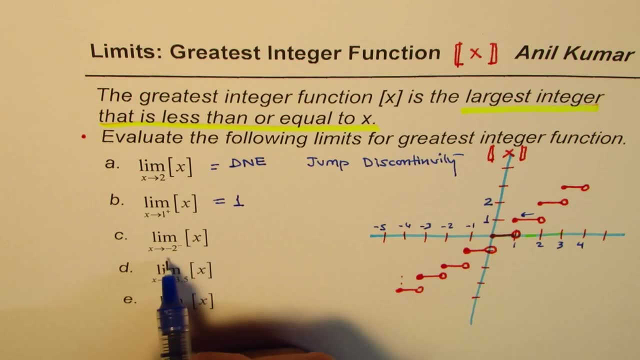 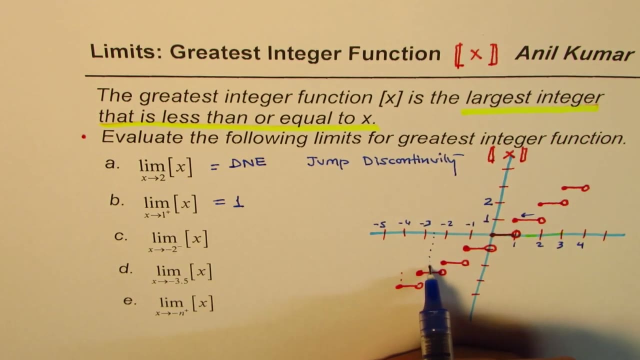 you're approaching one, so this is definitely one. is that clear? so you're kind of approaching from this side, so you're approaching one. then we have the limit of the function when you're approaching minus two from the left side. so minus two from the left side, you kind of here. so if I go kind of down here, I 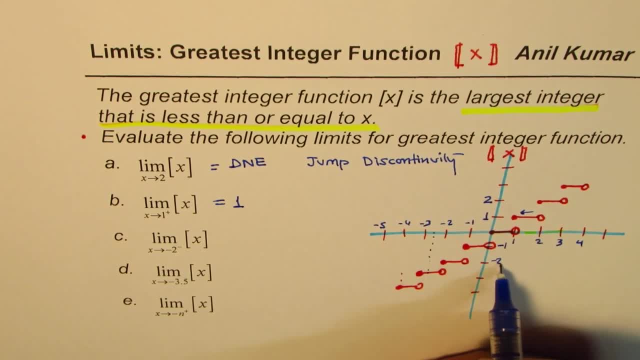 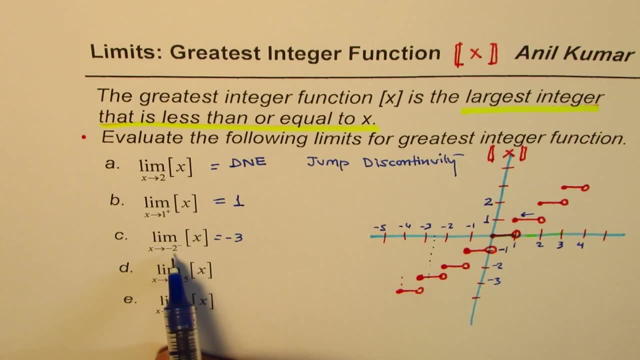 get to this value, which is minus one, minus two, minus three. do you see? so I get minus three, minus. so it makes sense. greatest integer lower than minus 2 is minus 3. right, all these numbers on a number line on the left side are lower. 1 is lower than 2. 0 is less than 1 minus 1 is less. 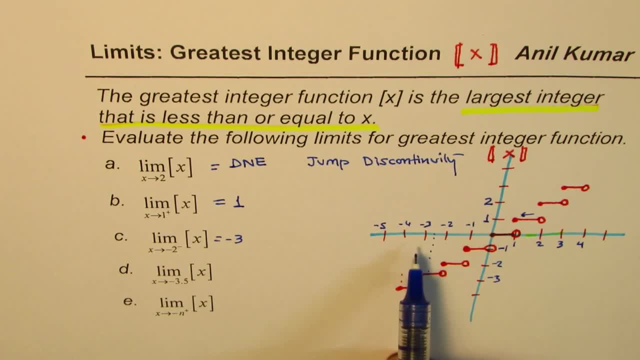 than 0. minus 4 is less than 3. you get the idea. now let's get to this one. it says limit of the function when x approaches minus 3.5, minus 3.5 somewhere here. so you are approaching this point from both the sides. either side, you approach a value of minus 4 and therefore this is minus 4. 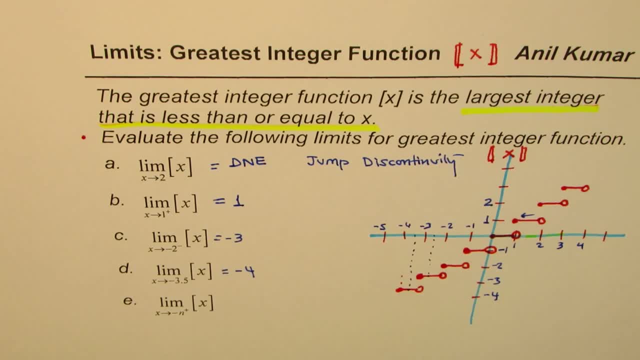 so, in between, you approach a value, but at the edge the limit does not exist. but if you are approaching from the right side, you see, you approach this value itself. n 1 b approach right, but if you are approaching from the left side, as we did for for two, you